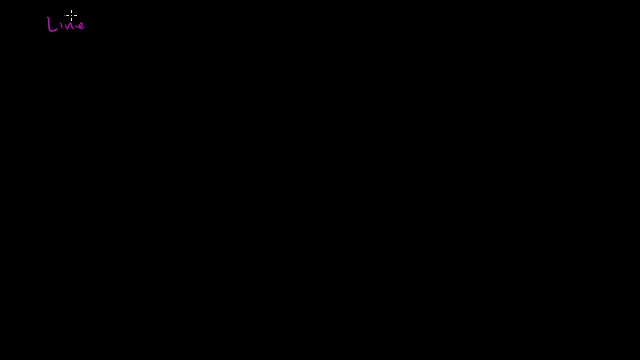 What I want to do in this video is think about the difference between a line segment, a line segment, a line, a line and a ray- And this is kind of the pure geometrical versions of these things, And so a line segment is actually probably what most of us associate with a line in our everyday lives. 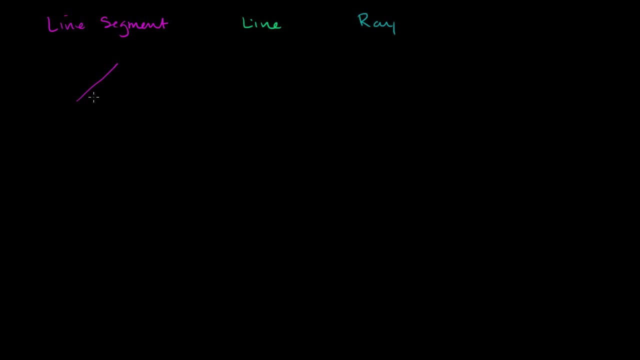 So a line segment is something just like that- for lack of a better word, a straight line. But why we call it a segment is that it actually has a starting and a stopping point. So most of the lines that we experience in our everyday reality are actually line segments. 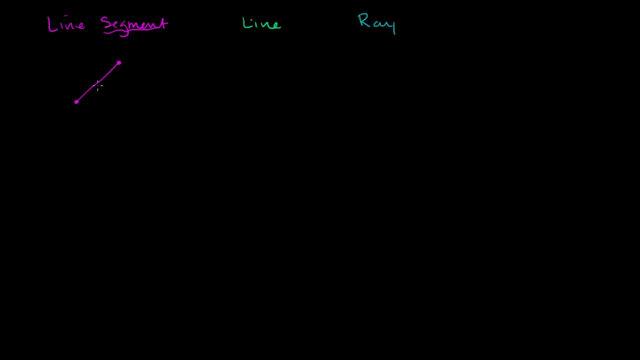 when we think of it from a pure geometrical point of view- And I know I drew a little bit of a curve here, but this is supposed to be completely straight. But it's a line segment. The segment is based on the fact that it has an ending point and a starting point. 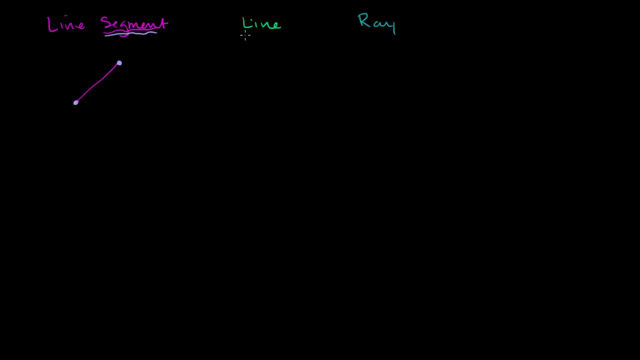 or a starting point and an ending point. A line, if you're thinking about it in the pure geometric sense of a line, is essentially: it does not stop, It does not have a starting point and an ending point. It keeps going on forever in both directions. 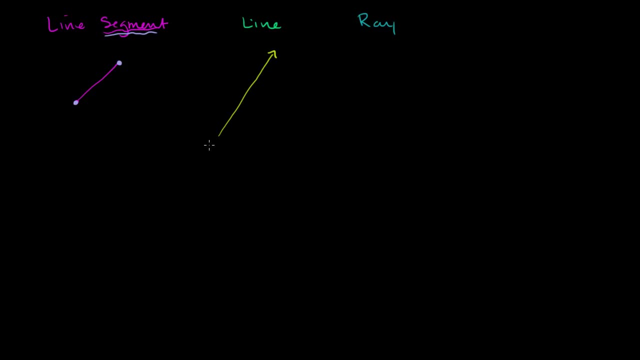 So a line would look like this: And to show that it keeps on going on forever in that direction, right over there, we draw this arrow. And to keep showing that it goes on forever in kind of the down left direction, we draw this arrow right over here. 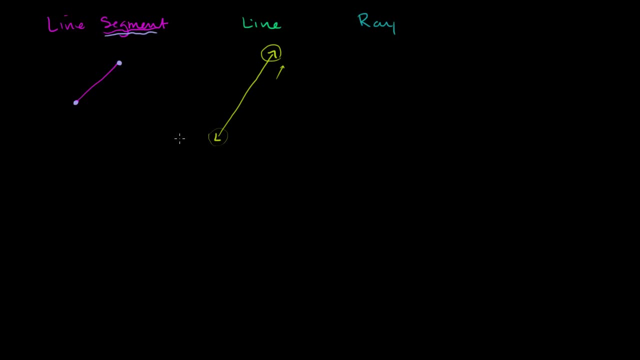 So obviously, you know, I've never encountered something that just keeps on going straight forever, forever. but in math- that's the neat thing about math- we can think about these abstract notions, And so the mathematical, purest, geometric sense of a line is this straight thing that goes on forever. 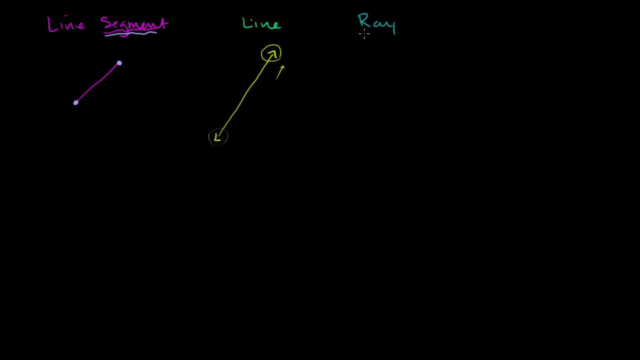 Now, a ray is something in between. A ray has a well-defined starting point, So that's its starting point, But then it just keeps on going on forever. So then, so the ray might start over here, but then it just keeps on going. 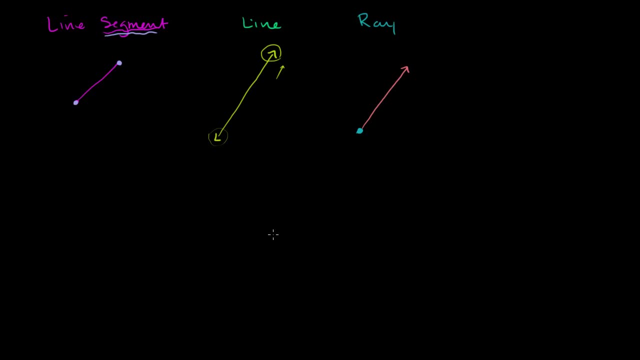 Then it just keeps on going So that right over there is a ray. Now, with that out of the way, let's actually try to do the Khan Academy module on recognizing the difference between line segments, lines and rays, And I think you'll find it pretty straightforward based on our little classification right over here. 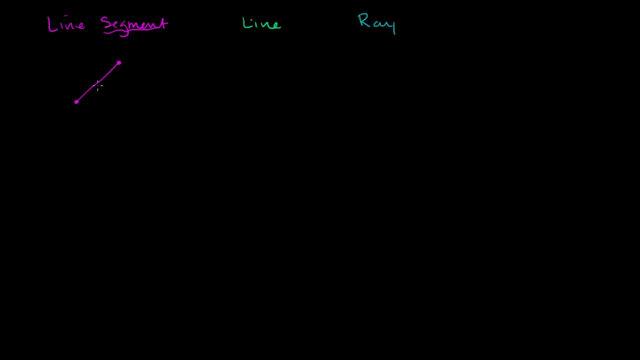 when we think of it from a pure geometrical point of view- And I know I drew a little bit of a curve here, but this is supposed to be completely straight. But it's a line segment. The segment is based on the fact that it has an ending point and a starting point. 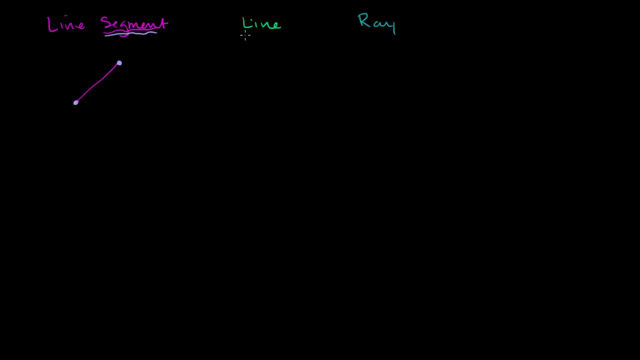 or a starting point and an ending point. A line, if you're thinking about it in the pure geometric sense of a line, is essentially: it does not stop, It does not have a starting point and an ending point. It keeps going on forever in both directions. 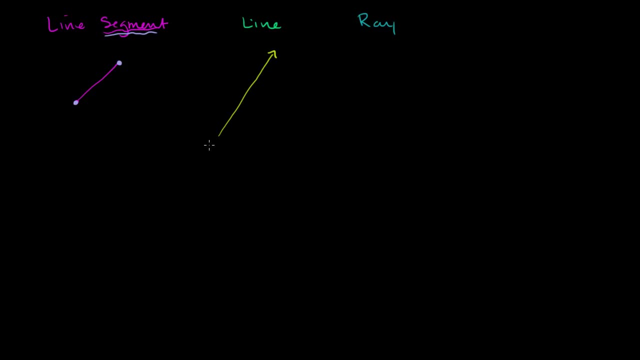 So a line would look like this: And to show that it keeps on going on forever in that direction, right over there, we draw this arrow. And to keep showing that it goes on forever in kind of the down left direction, we draw this arrow right over here. 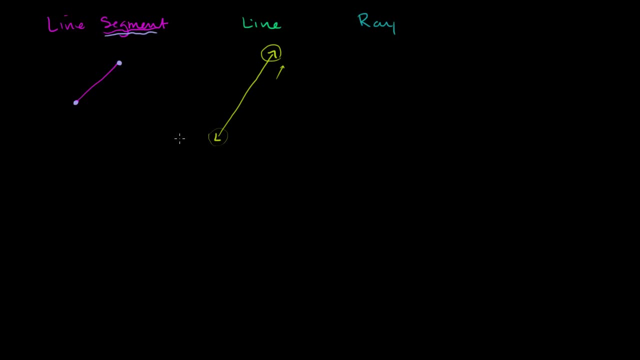 So obviously, you know, I've never encountered something that just keeps on going straight forever, forever. but in math- that's the neat thing about math- we can think about these abstract notions, And so the mathematical, purest, geometric sense of a line is this straight thing that goes on forever. 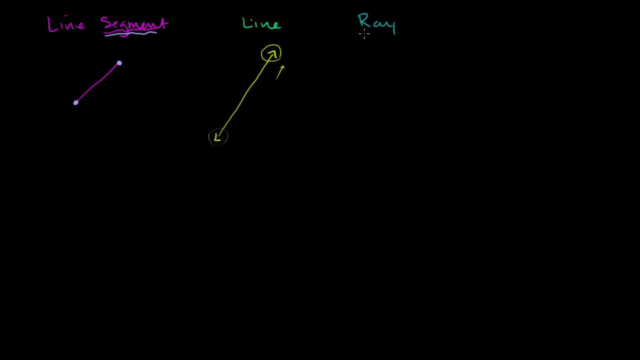 Now, a ray is something in between. A ray has a well-defined starting point, So that's its starting point, But then it just keeps on going on forever. So then, so the ray might start over here, but then it just keeps on going. 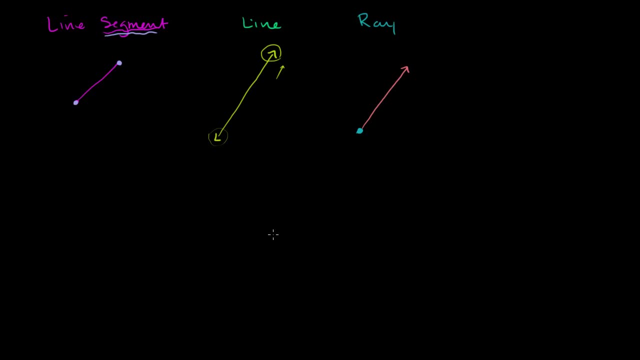 Then it just keeps on going So that right over there is a ray. Now, with that out of the way, let's actually try to do the Khan Academy module on recognizing the difference between line segments, lines and rays, And I think you'll find it pretty straightforward based on our little classification right over here. 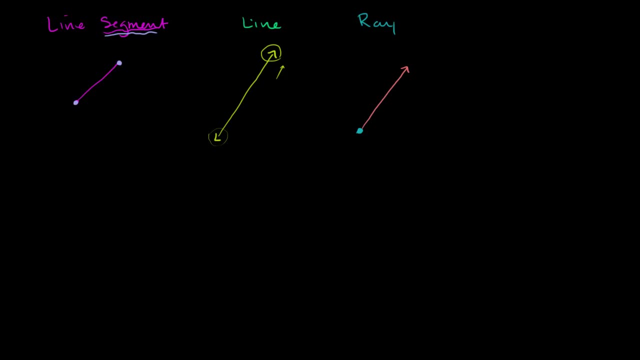 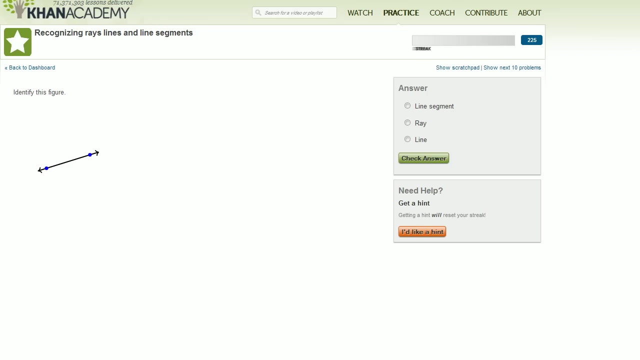 So let me get the module. let me get the module going. Let me let me, where did I put it? Where did I put it? There you go, All right. So what is this thing right over here? Well, it has two arrows on both ends. 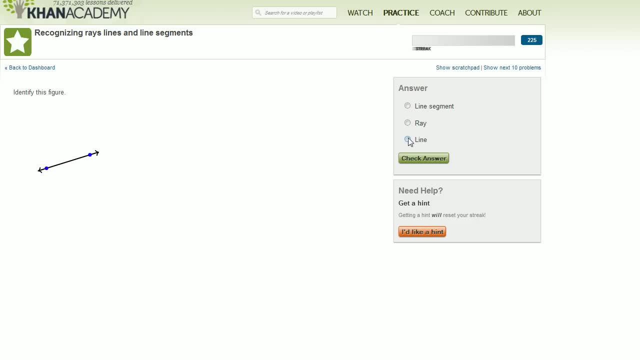 So it's implying that it goes on forever. So this is going to be a line. Let's check our answer. Yeah, it's a line. Now it's taking some time. I'll correct next question. All right, Now what about this thing?